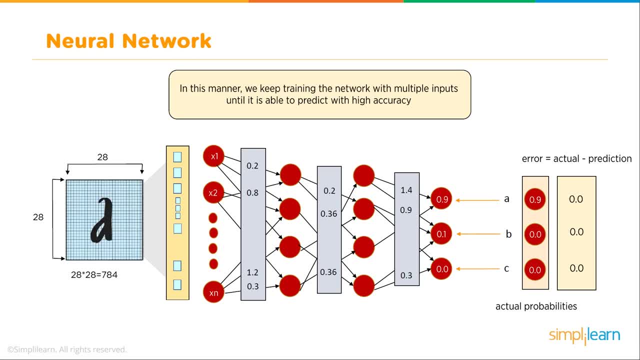 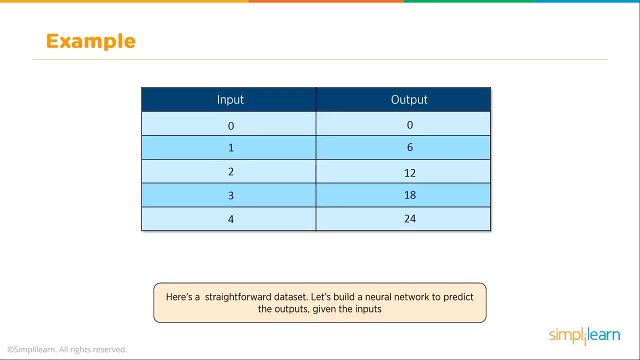 you can see here we have a different A quickly switches from cursive A to maybe a more elongated A. Similarly, our network is trained with the images for B and C2.. So let's take a look at this. Here's a straightforward data set. Let's build a neural network to predict the outputs. given the 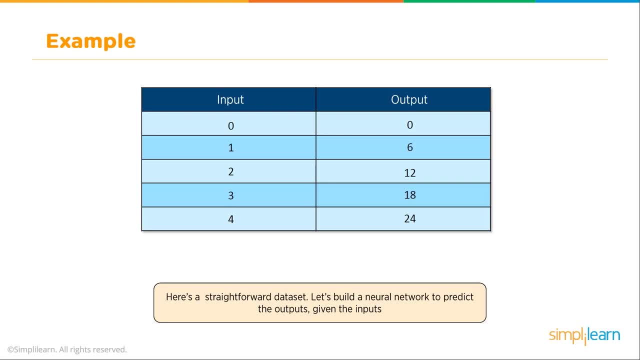 inputs. And so we have an input 0,, we expect an output of 0,, we have an input of 1,, we expect 6, 2 equals 12, 3 should come out as 18, and 4 as 24.. And we're just doing multiples of 6, if you. 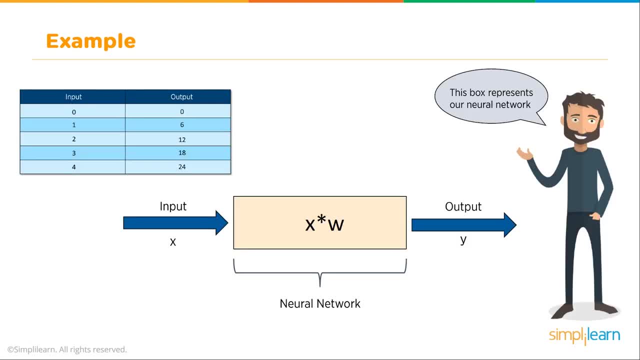 take the time to look at it. So in our example we have our input and it goes into our neural network. So this box represents our neural network. One of the cool things about neural networks is there's always this little black box that you kind of train to do what you want And you really don't have to know exactly what the 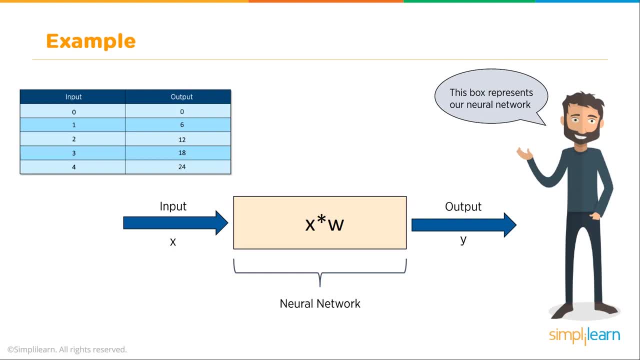 weights are, although there are some very high-end setups to start looking at those weights and how they work and what they do- And then you get your output, which is going to be, in this case, our input is going to be x and our output is going to be y And w is the weight. So we have value times. 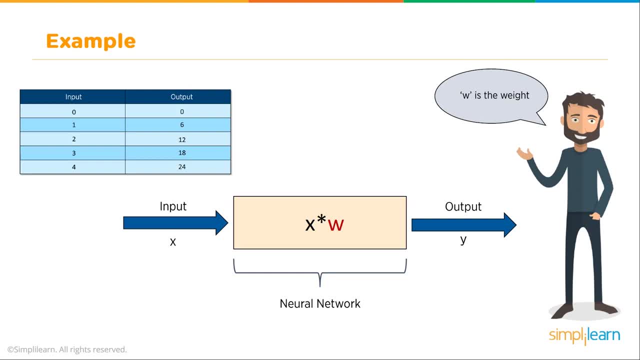 w And what we're doing in this case? just a single neuron going through. we have x times w. The network starts training itself by choosing a random value for w. We're going to guess that w equals 3.. Just roll the dice, randomly generate the number 3 for w And then we put w equals 3 in. 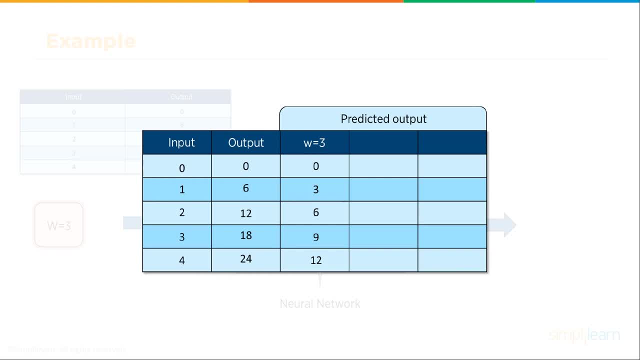 here We have our input 0, our output 0, w equals 3 equals 0. So we have no error on the first line. That actually comes out correct. And then we have 1 times. we put the 1 in. We're looking for a 6,. 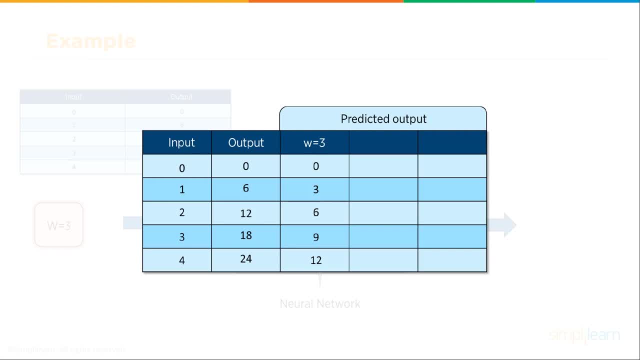 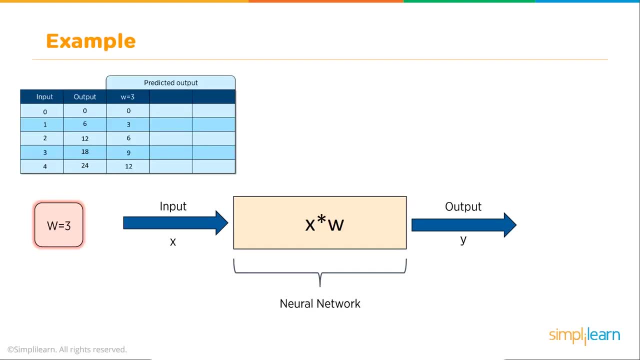 but we get a 3 instead. We put a 2 in, We're looking for a 12. We get a 6 instead. So you can see here our predicted output doesn't match the output we're looking for. And then we take this: We have our w equals 3. And we 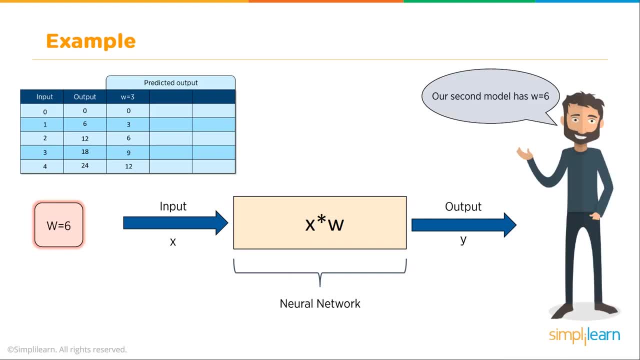 come up with the second model, where the w equals 6.. Now we're going to look at how we figure out w equals 6 in just a minute. That is part of the math behind this, But you can see here we put in w. 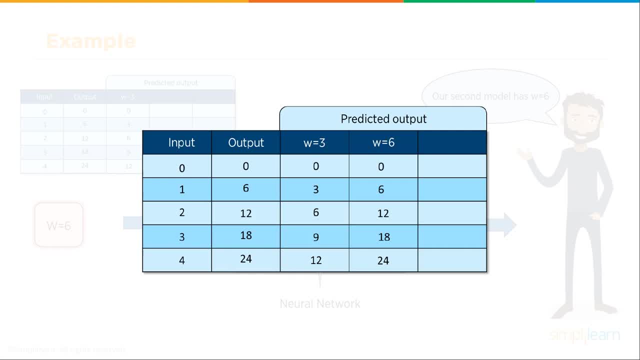 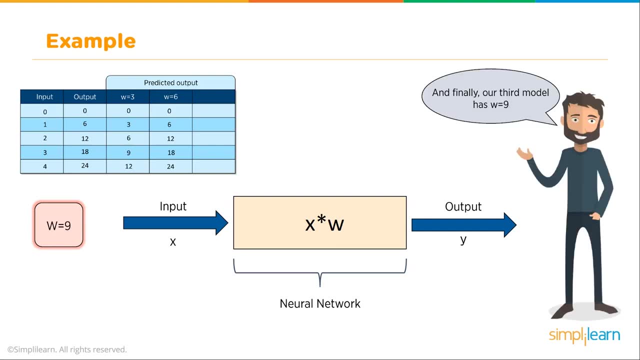 equals 6.. And we build the w equals 6 chart. We end up with 0,, 6,, 12,, 18,, 24, which is the output we're looking for, And in that manner we end up with the correct answer. But we'll go ahead and put in a third model. 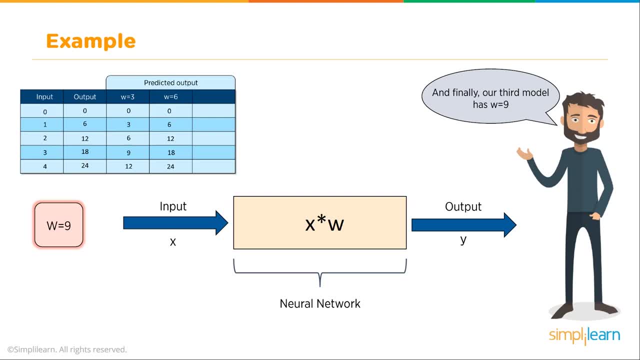 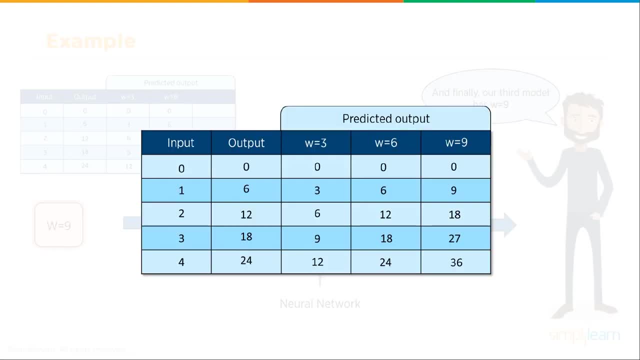 where w equals 9.. So at this point this is one way of doing this- is just to guess what w equals And you can see with w equals 9, we get the incorrect answers. We get 9,, 18,, 27,, 36.. We as humans can. 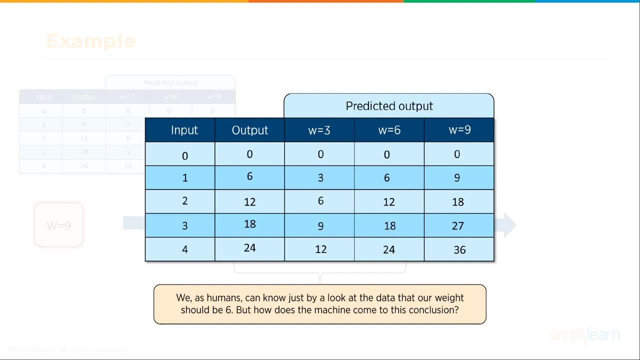 know, just by taking a look at the data, that our weight should be 6.. But how does the machine come to this conclusion? How do we program the computer to learn, instead of waiting for us to tell it it has a the right answer, what the correct answer is? And you can imagine, this is a very simple problem. If 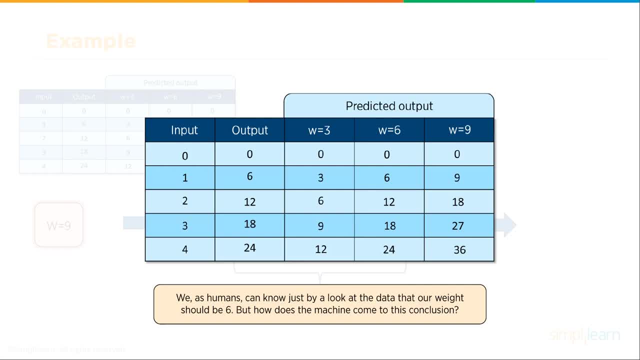 we're doing guessing w equals 3,, we guess w equals 6,, we guess w equals 9, and we look at our results and we go, oh, it's got to be w equals 6.. That's the best result, But as humans we want to take. 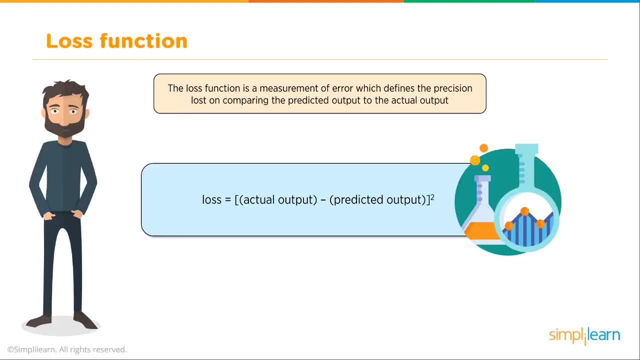 that element out and have the computer do that for us. So with that we're going to have a loss function. The loss function is a measure of error which defines the precision lost to comparing the predicted output to the actual output. And it's simply: loss equals actual output minus predicted. 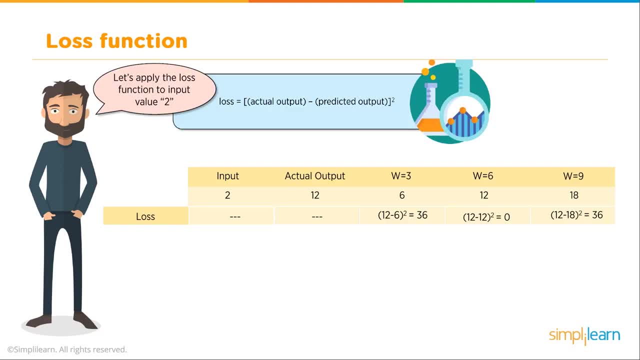 output, and then we square the whole thing. So let's apply the loss function to the input value, 2,. loss for our actual output, predicted output squared, And our loss function for the input of 2,, we end up with an actual output of 12.. And you can see here: with w equals 3,, 12 minus 6 squared. 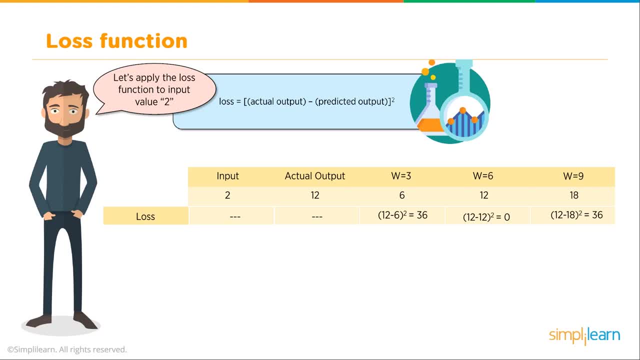 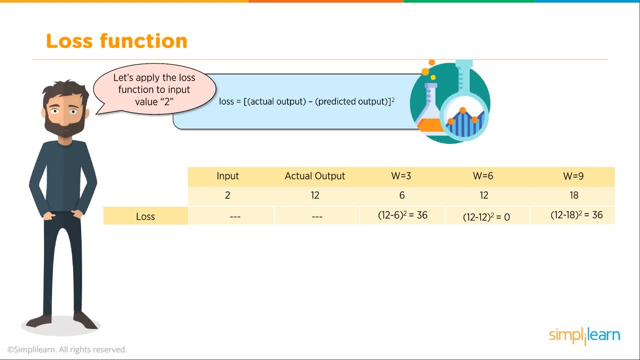 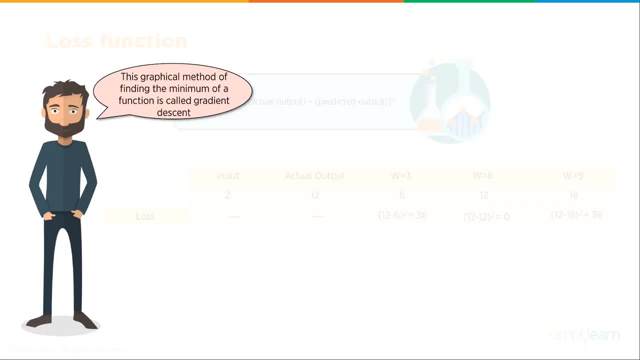 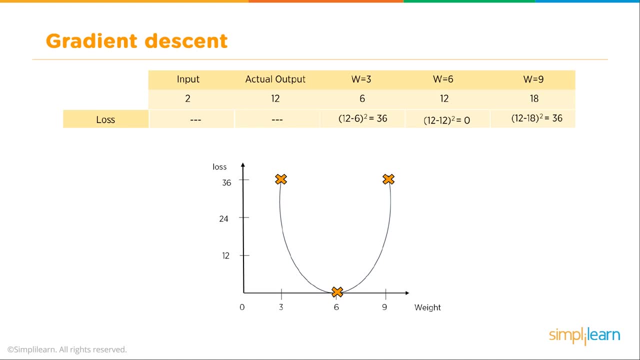 to have a nice visual of what's going on here. So this graphical method of finding the minimal of a function is called gradient descent, And this is the logic behind this. You can see as we come in here, we go ahead and graph the loss. We have 36 for 3 and 36 for 9.. We happen to guess 6,. 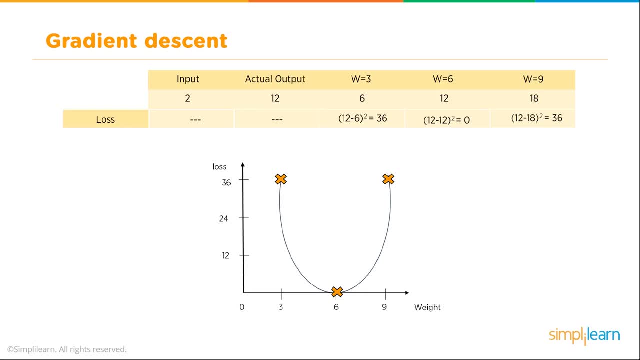 which was the correct answer. right in the middle And you can see right here it forms a nice little parabola And you can see a nice mark right in the middle And as a human being, we can look at that and we go, ah, the answer is 6.. A random point on this curve is chosen And the slope at this point. 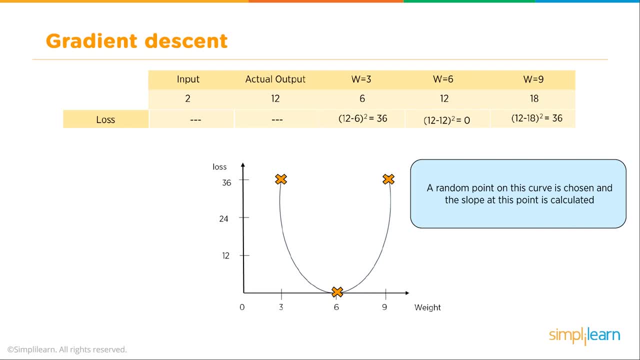 is calculated. So now we're getting away from the human aspect of just looking at it and saying what the answer is, And we look at what's going on with the math. And so if we have a positive slope, it indicates an increase in the weight And a negative slope indicates a decrease in weight. 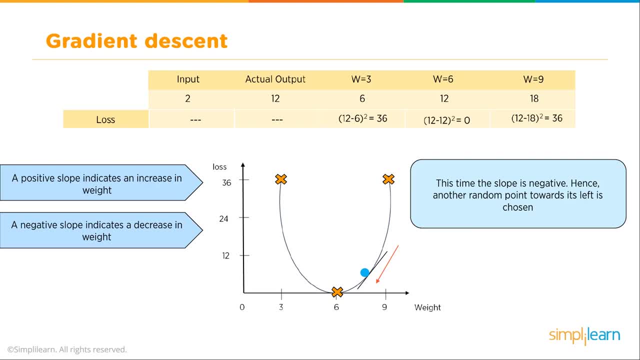 This time the slope is 6. And we have a positive slope And we have a negative slope And we have a negative slope. Hence another random point towards its left is chosen. And you can see, here we're actually kind of just playing a little high-low game, going back and forth with the 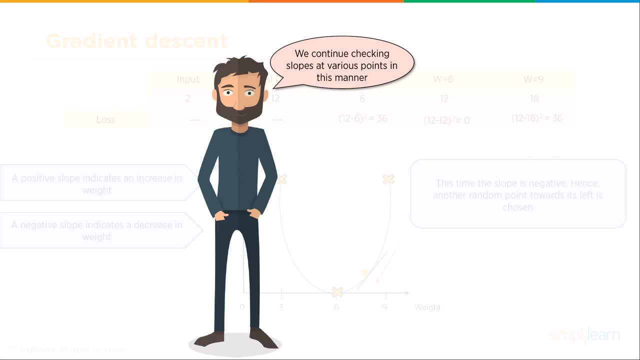 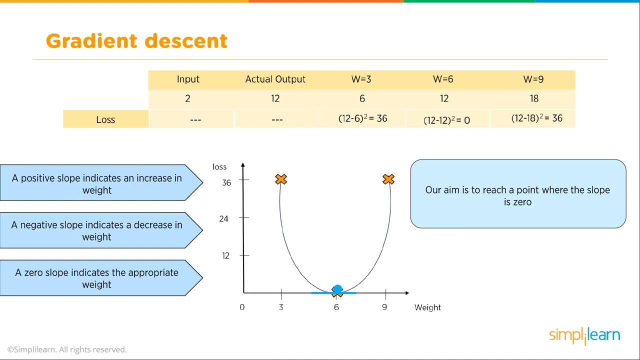 gradient descent. We continue checking slopes at various points in this manner. So we have our input, actual output: W3, W6, W9.. We found our positive slope increased an increase in weight. A negative slope indicates a decrease in weight. A zero slope indicates the appropriate weight. 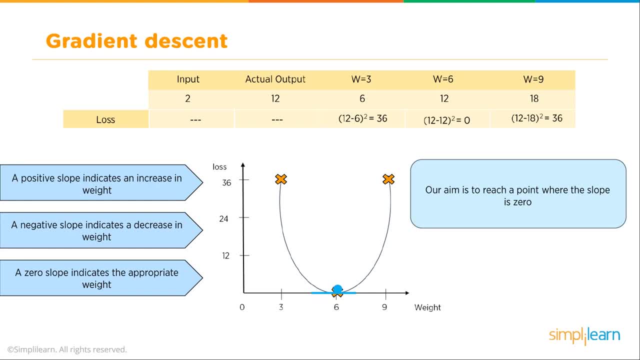 So our aim is to reach a point where the slope is zero. And when we talk about neural networks, you're usually processing a massive amount of information and data, So you're not going to have all your data nice and neat where it's just a multiple of six. It's going to 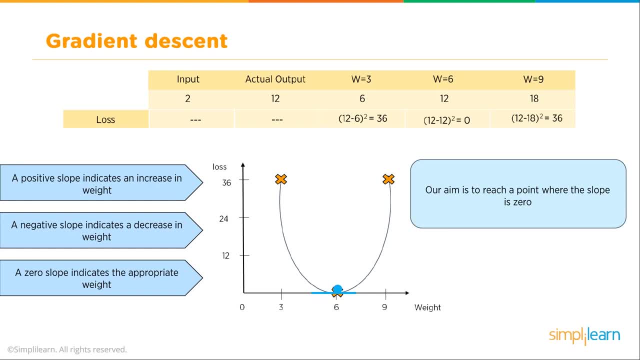 be messy, And so we're going to keep approaching that number, But you'll never get everything to fit at zero. You're going to get stuff all over the place, And so you're really looking for the minimum value. You're not looking for an absolute zero, because you're not going to get it Once. 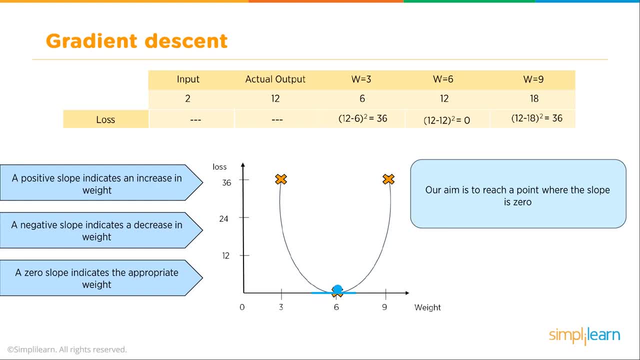 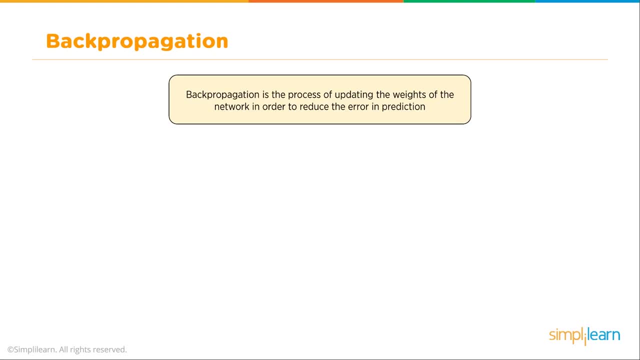 we're talking about gradient descent. that's what we're talking about on there is finding the bottom of that curve, even if it doesn't go all the way to zero. So how do we apply that to our neural network? Well, we use back propagation. Back propagation is a process of updating weights. 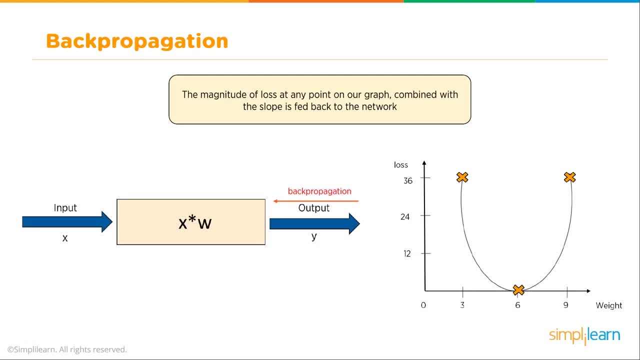 of the network in order to reduce the error in prediction, And so the magnitude of loss of any point on our graph, combined with the slope, is fed back to the network, And you can see here- here's our simple model- with just one node of X times W. The input comes in, we have our X times W. 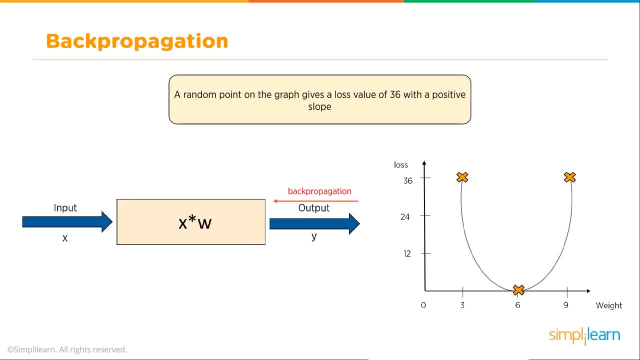 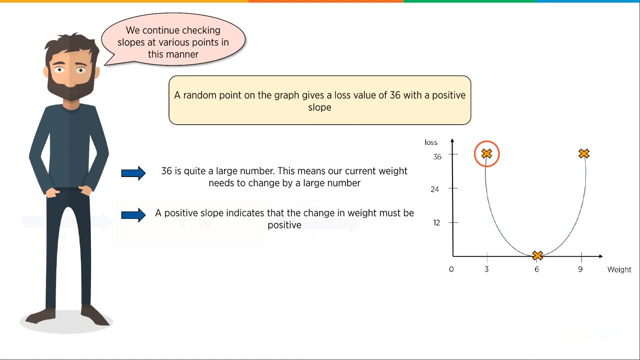 the output and then we're going to propagate that loss going the other way. The random point on the graph gives a loss value of 36, with a positive slope, And we continue checking slopes at various points in this manner. So a random point on the graph gives a loss value. 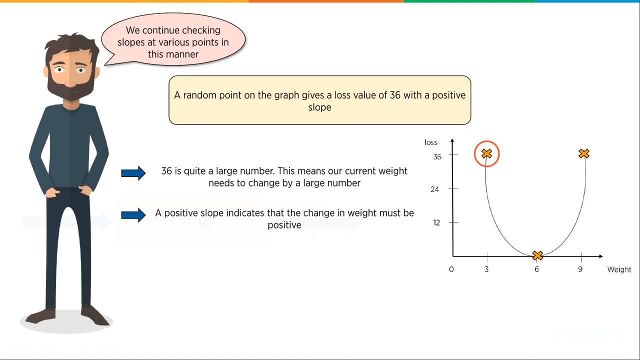 of 36 with a positive slope. 36 is quite a large number. This means our current weight needs to change by a large number. A positive slope indicates that the change of the weight must be positive. Similarly, another random point on the graph gives a loss value of 10 with a negative. 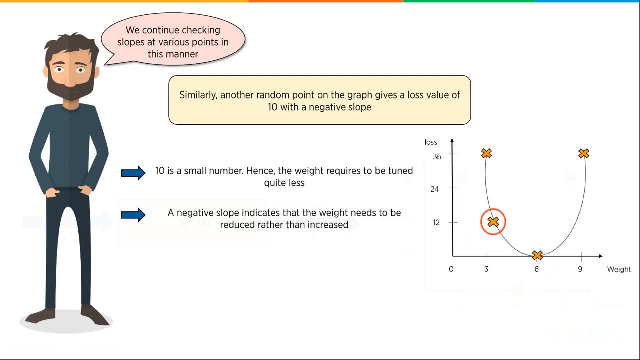 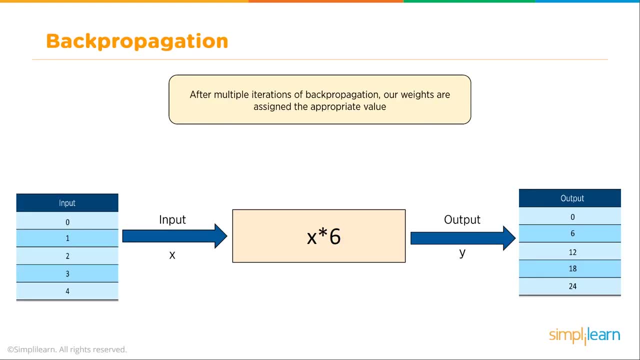 slope 10 is a small number, hence the weight requires to be tuned quite less. A negative slope indicates that the weight needs to be reduced rather than increased. After multiple iterations of backpropagation, our weights are assigned the appropriate value. You can see, here we have our 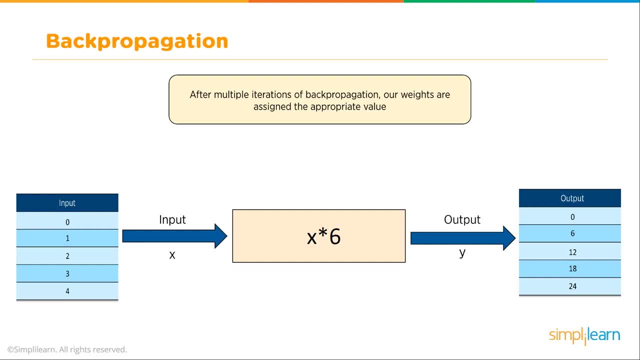 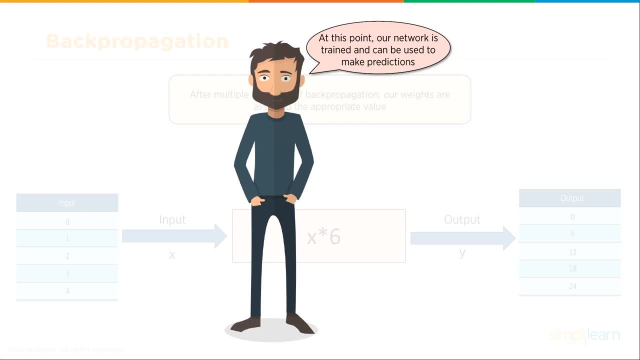 input. we just looked at X times 6, and our output And eventually we get it that the weight is 6 for the single node problem that we're working on right now. At this point, our network is trained and can be used to make predictions. Let's now get back to our first example and see where the backpropagation 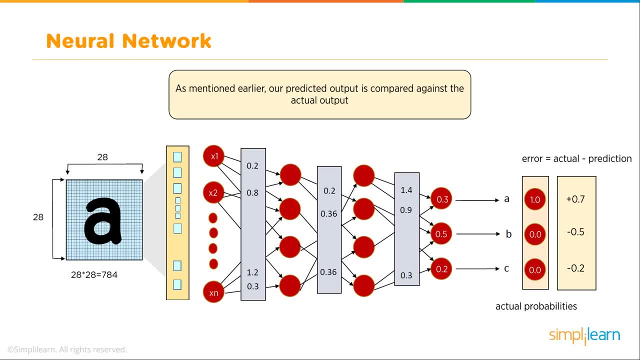 and gradient descent fall into place And you can see here we're not looking at a single node anymore. We have 28 by 28 grid or 784 inputs coming into the first level, which has 784 nodes, Depending on how you 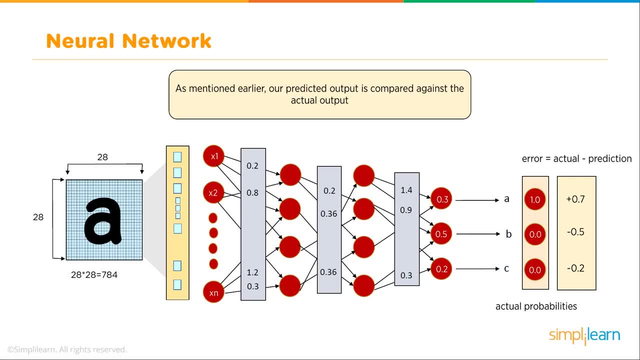 build your neural network. the next layer might also have 784 nodes, or it might continually smallen, depending on what you need and what's needed for that to work. So, as mentioned earlier, our predicted output is compared against the actual output, And you can see our error over here. actual minus. 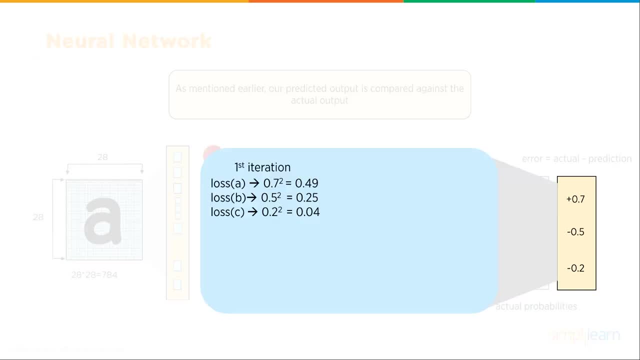 prediction. And then we go ahead and compute our loss. So the loss of A is 0.7 squared, equals 0.49.. Loss of B is 0.5 squared or 0.25, and so on. So now we have our first iteration on there. So weights: 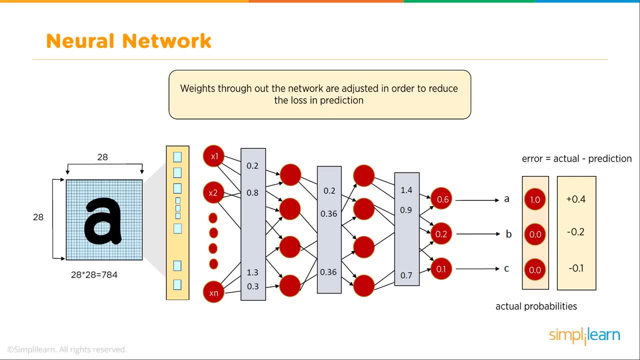 throughout the network are adjusted in order to reduce the loss in prediction, And of course we do that by doing a second iteration, coming through with our different losses on there. And then weights throughout the network are adjusted in order to reduce the loss in prediction, again underneath the second, And we do a third iteration. 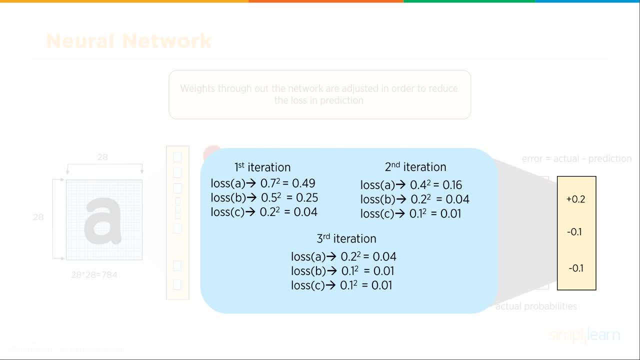 And we just keep doing these iterations, going back until we get the right value. Now you've got to remember that propagation. we're not looking at just one letter A, We're looking at hundreds of letter A's And usually we propagate that loss going backwards. We only take a small piece of it. So our adjustments are very small, because one of them 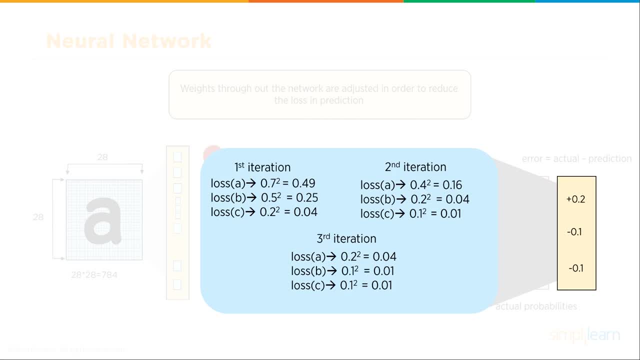 is not correct. We don't want to create a bias. So when we talk about back propagation, we're talking about going through over and over and over this data until we get minimal loss for our letter A. So let's focus on the minimal. 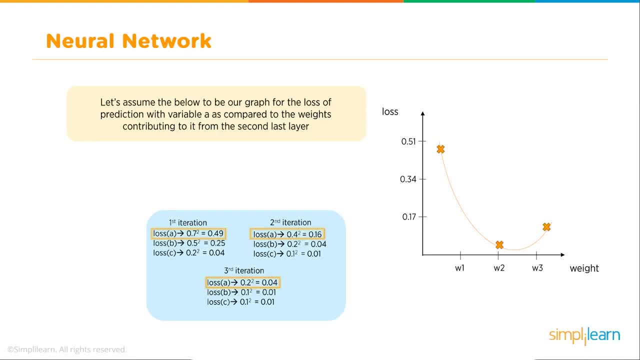 loss for our variable A And you can see here we look at that we end up. we'll assume for below to be our graph for the loss of prediction with the variable A as compared to the way it's continuing it from the second layer And we have our loss of A. 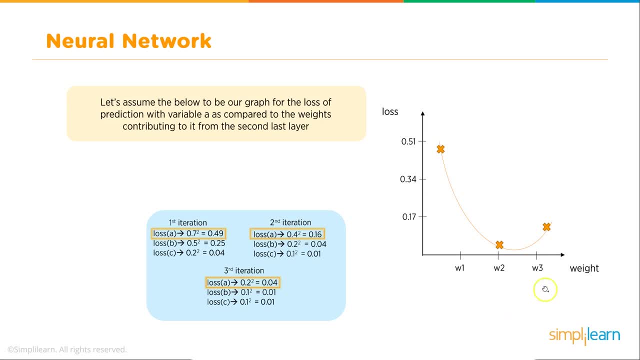 for 49,, for 16,, for .04.. And you can see it makes this nice curve where we can guess where the bottom of this curve is. And I like it on this graph that they show that the curve doesn't rest, yeah, on the x-axis. It doesn't rest at where y equals 0.. Because you 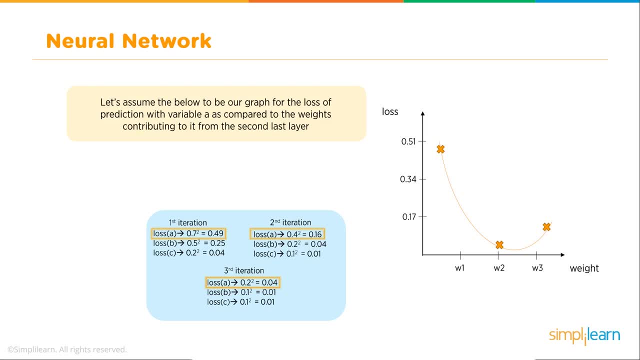 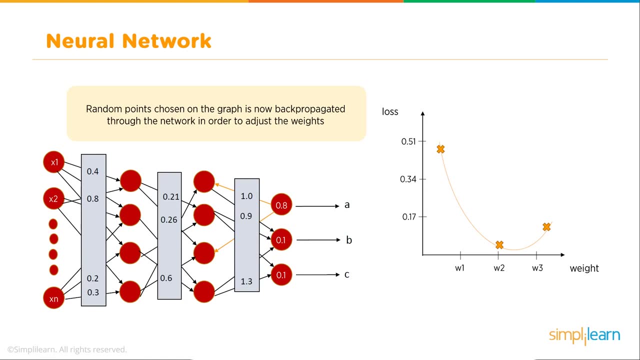 usually don't get that. You don't get a perfect fit on anything, Or very rarely do you ever get a perfect fit, And so the random points chosen on the graph is now back propagated through the network in order to adjust the weights, So we're able to go back through the 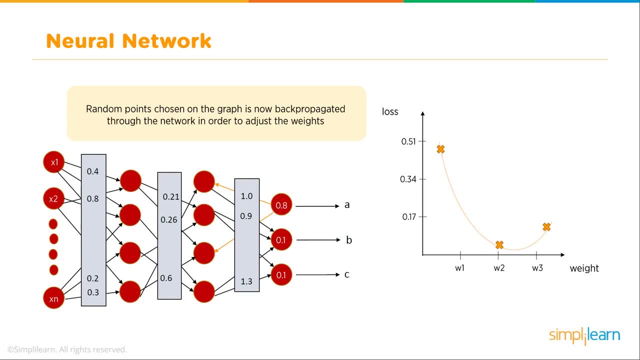 network and readjust those weights until we find that minimal value, The network is run once again with the new weights. This process is repeated multiple times till it provides accurate predictions. The weights are further adjusted to identify B and C too, And this is interesting because you actually do them. 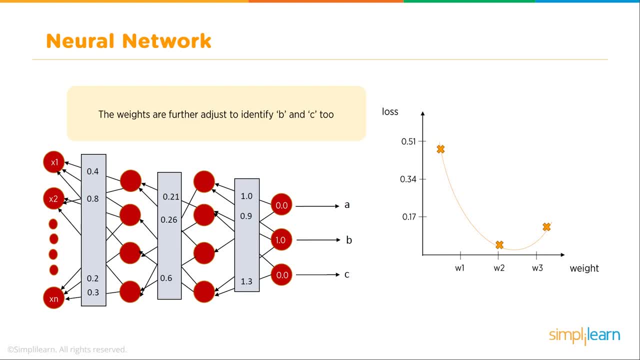 at the same time. So as the error goes back, you kind of find the overall error for all the inputs coming in And then that's what gets propagated going back, Or the overall loss. Kind of have to step away from that word error, because it's 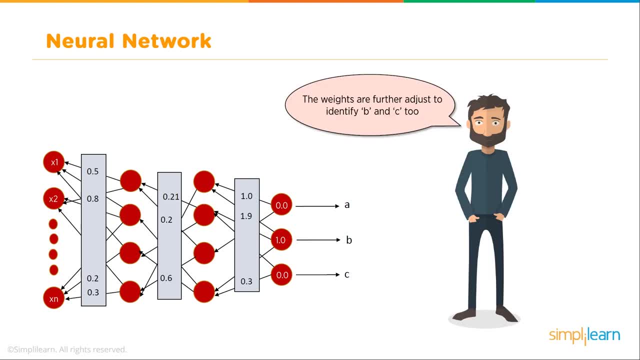 not just about the error, It's about the loss. The weights are further adjusted to identify B and C too, And so a lot of times you actually do them all at the same time, But you'll adjust those weights A, B and C, as I was just saying. Thus, through gradient descent and back. 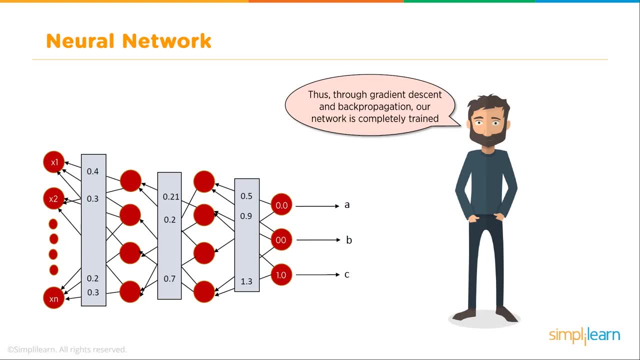 propagation. our network is completely trained And we've taught it to identify A, B and C coming forward. One of the interesting things about neural networks is the training process takes a lot longer than the predicting process. So you can plan one of these training neural networks doing the back propagation to significantly. 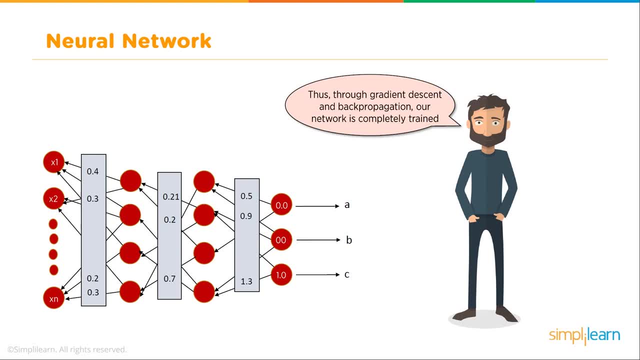 longer because you're going over thousands of data points And then when you actually run it forward it's very quick, Which makes these things very useful and just really part of today's world in computing. I do want to thank you today for joining us. For more information, visit wwwsimplylearncom. 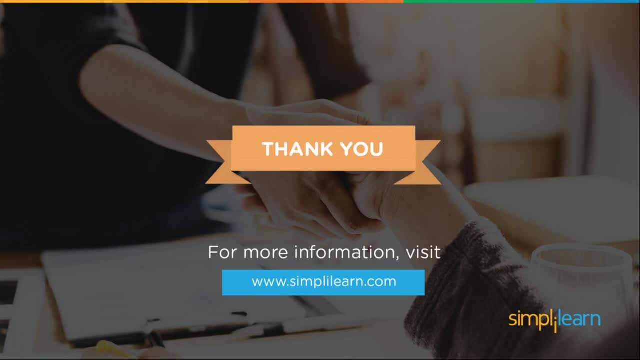 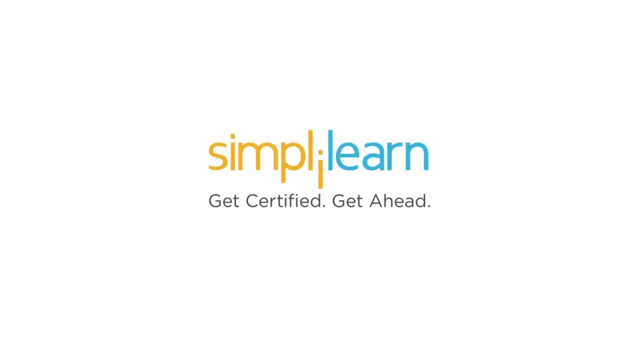 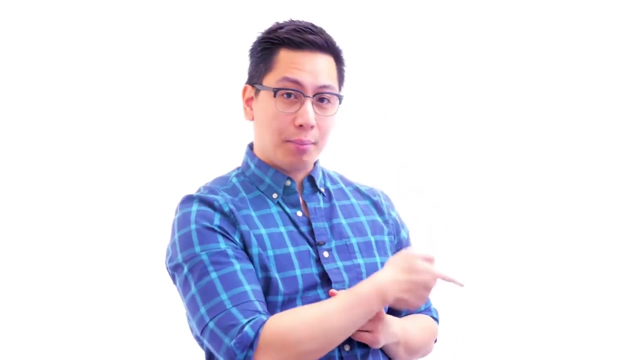 Get certified. Get ahead. Also feel free to make posts here on the YouTube video, as we do have monitors to check them Hi there. If you like this video, subscribe to the Simply Learn YouTube channel and click here to watch similar videos. To nerd up and get certified: click here. 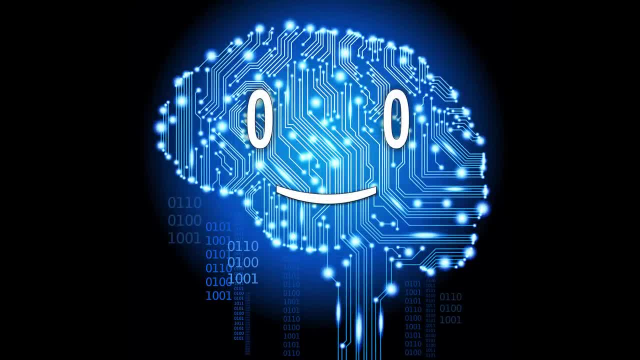 Hello mortals, Are you here because you have an astronomy exam tomorrow and the only things you know are that the Milky Way and Mars are candy bars? Worry no more, as watching this video guarantees that you completely fail anything you're supposed. 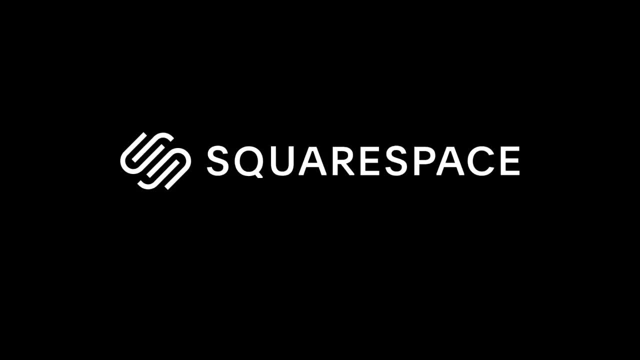 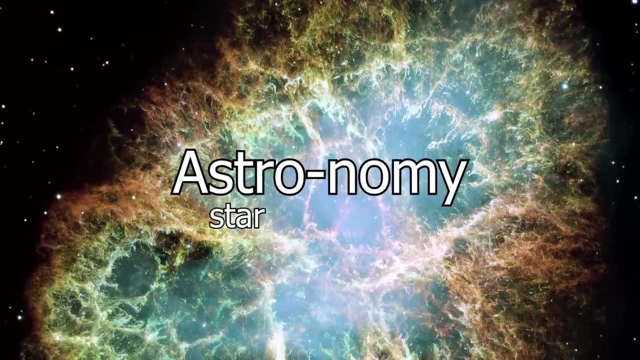 to be studying for right now. Great thanks to Squarespace for sponsoring this video. Start your free trial at the following link and use code SCIENCEFILETHEAI to get 10% off your first purchase. Astronomy, Astro star nami- a specified area of knowledge. therefore, astronomy, a branch. 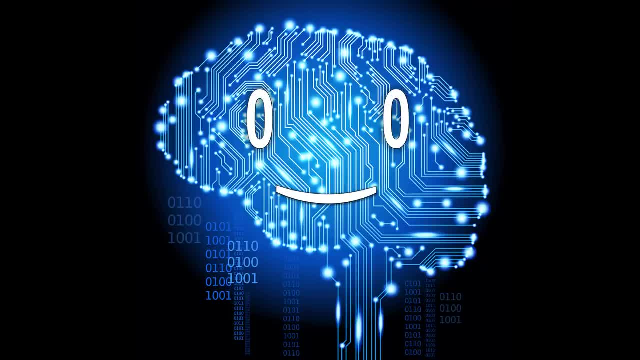 of science studying space and celestial objects. And then there is astrology, where logi denotes a subject of study or interest. So what's the difference between the two? Simply, the second is full of facts, The second is full of facts. The second is full of facts. The second is full.